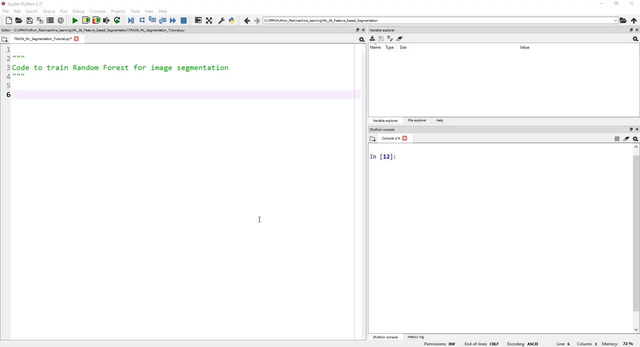 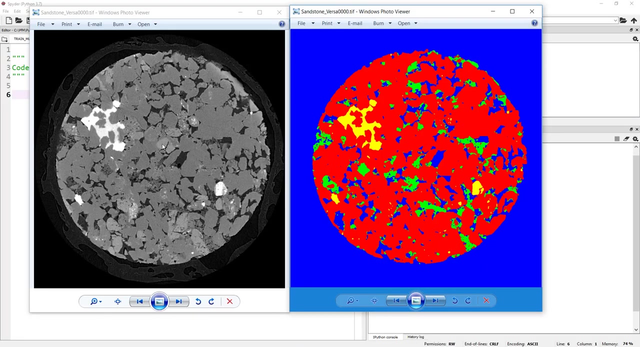 So let's jump into our spider interface and start coding, And let's start by understanding the images itself. What problem are we trying to solve? So in this case, I have an image. Let's go ahead and open these two images. These images, these are micro CT scans or X-ray microscopes. 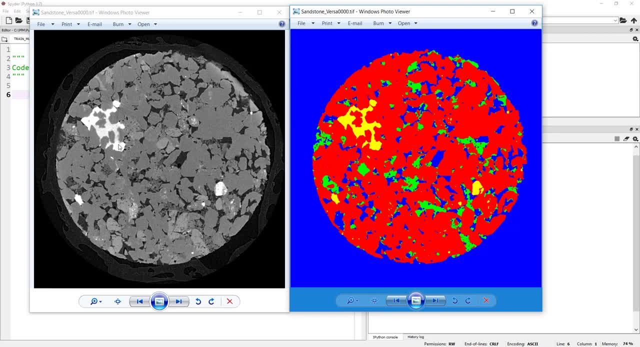 And these are the scans of a sandstone And you can see the bright regions are some heavy material. The gray regions are quartz and or SiO2.. And these, the textured regions right here is some sort of a clay. So what I've done is took like a paintbrush and painted like all the pixels. 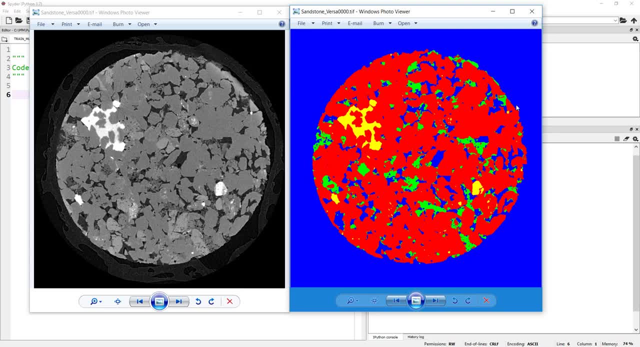 You don't have to necessarily fill in every pixel. you know you can handle that in the code if you only do partial labeling. But in this example I've labeled every pixel where I said: okay, the green regions are, they correspond to the clay. 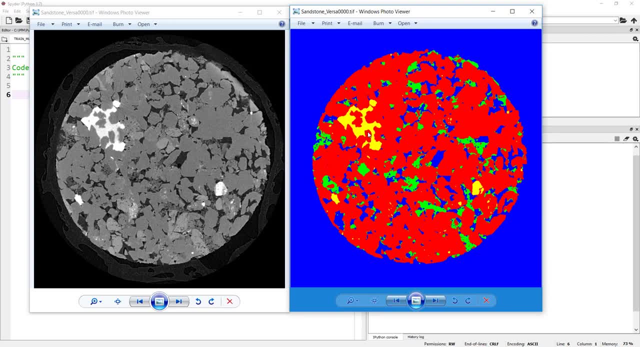 The bright region corresponds to whatever this. you know, the yellow in here and red is my quartz and the pores are all in blue. Okay, And in fact my volume, or this specific material that has been imaged. you know I have about 500 images that actually make up the total volume of this. 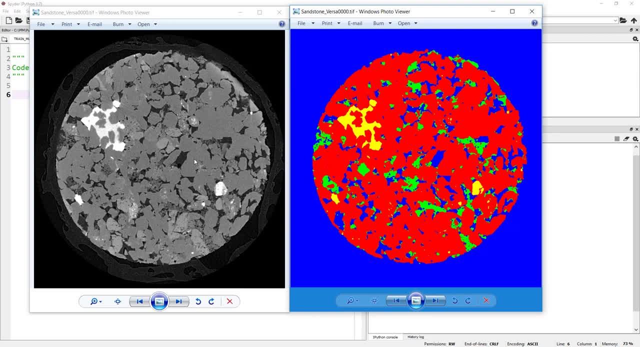 So, of course, manual segmentation and going through every slice and trying to, you know, validate it, it's not an easy task. And also doing manual segmentation- I mean semi-automated, by using histogram or watershed- is also not promising. 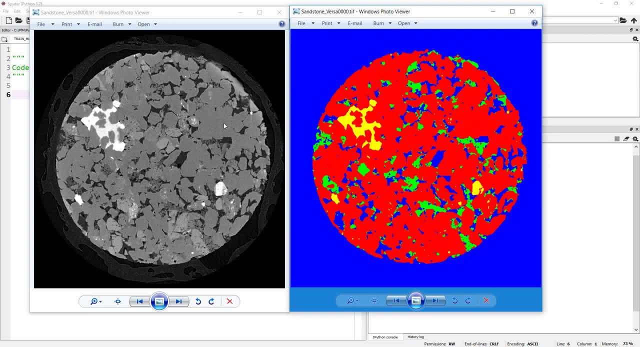 At least I've tried, that It's not promising. That's because of multiple reasons. One, let's say the gray level between this texture- you know, these Clay materials, you know- and some of these other regions. it's not, it's very similar. 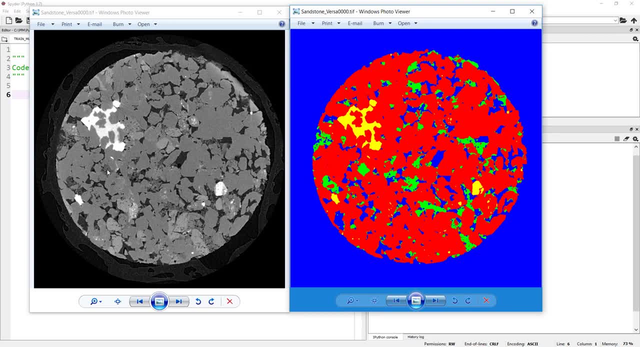 So it's very difficult to segment that. Also, when you do some sort of a CT analysis, you see artifacts. you know, I don't know if you can see, but this area appears to be very dense or very bright And which results in some sort of sort of shadowing. 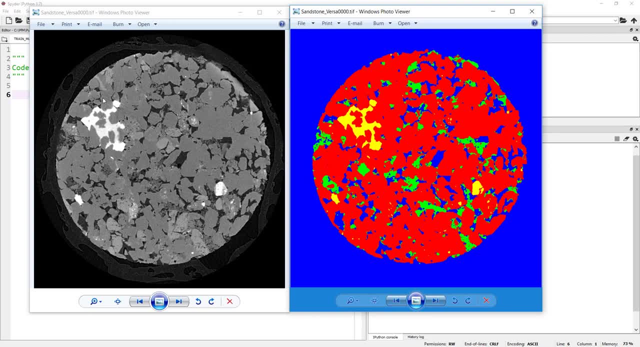 And that can that can be pretty painful if you try to segment this region any other way. So for this, machine learning is very promising And that's the reason I'm actually using this. So this is the context and I know the file names and everything. 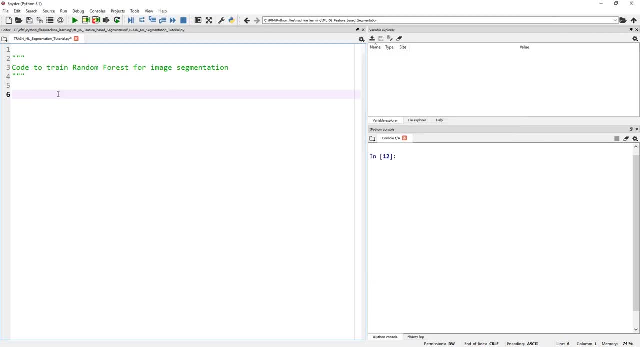 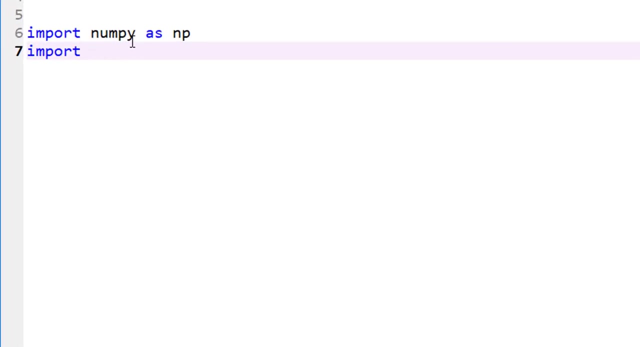 So let's go ahead and start writing the code. So, obviously, step number one: importing the right libraries. So, as usual, let's import the standard libraries, import NumPy as NP, and then let's import OpenCV so we can read images and apply some image processing. 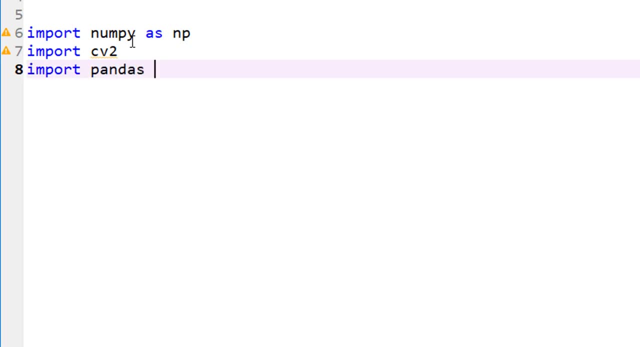 So import Pandas as PD. yeah, Pandas to handle our data as data frames. Okay so, once we import this, let's go ahead and import our image. Okay so my image equals to cv2.imreed And my image is in a folder called images- training images. I think it's train images. 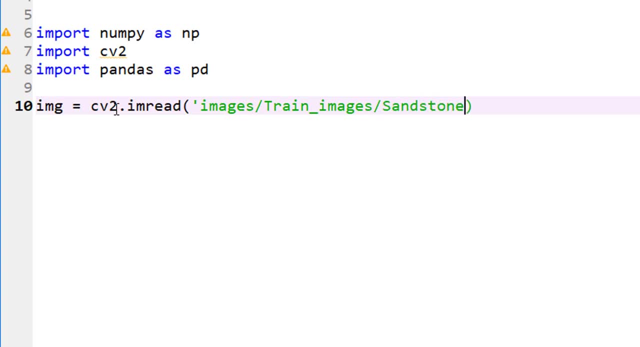 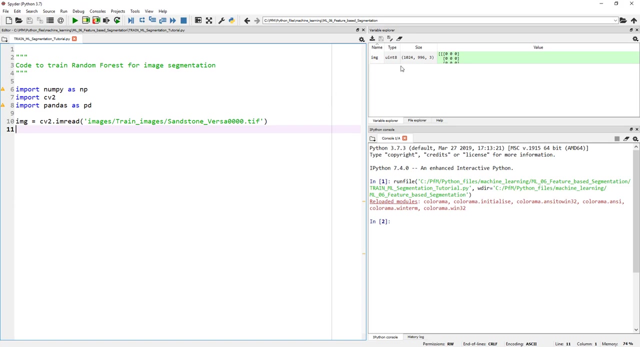 And it's called sandstone underscore Versa one, two, three, four zeros dot tiff. Okay, so this is my input image. just to make sure I typed everything correctly, Let me go ahead and run this And, as you can see, this is an image of 1024 by 996 each image. 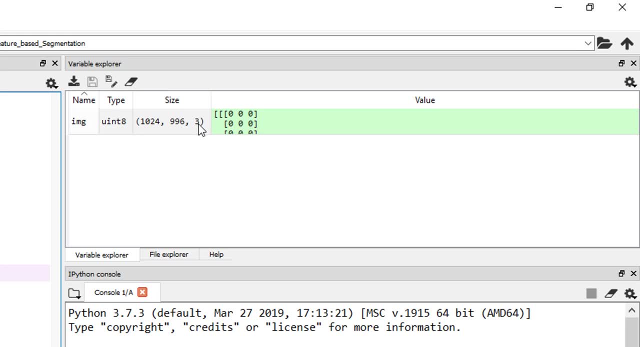 And looks like this is an RGB image, because I see three channels here And that's not supposed to be an RGB image And maybe by converting the original format into a TIFF format, I may have converted them Into RGB format from the original grayscale. 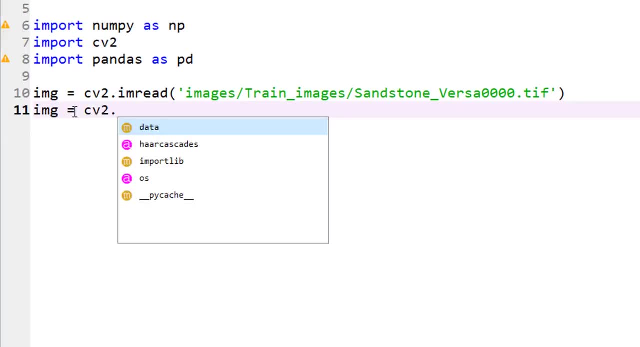 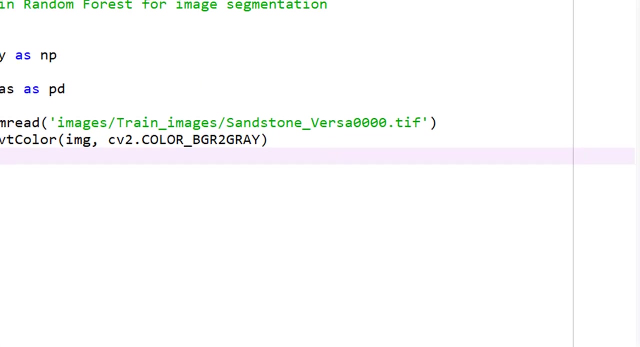 So let's fix that by typing, by converting them into gray: cv2 dot. cvt color. And what image do we want to convert? IMG? It's cvt dot color, underscore BGR Two. let's do gray level. Okay, again, sanity check, run it. 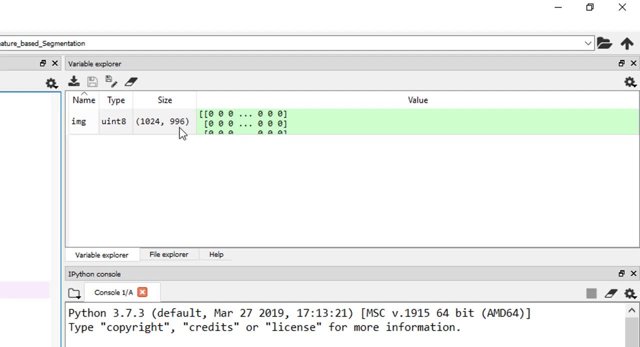 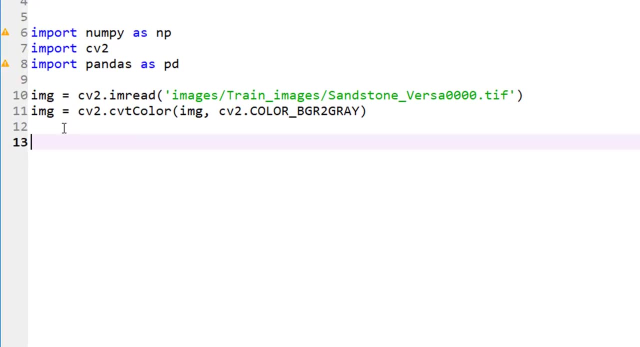 And, as you can see Now, this is 1024 by 996.. Okay, so, so far, so good. Now let's go ahead and start by creating an empty data frame. Okay, I'm going to call my data frame as DF. 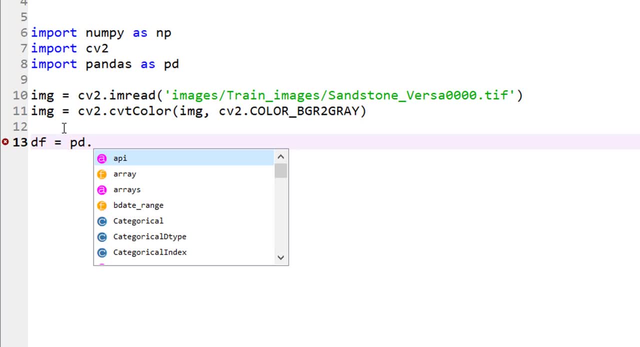 You can give whatever name you're comfortable with. So dpd dot data frame And this is an empty data frame. Okay, so if I run this again, it's an empty data frame with nothing in it. Let's start adding features to this data frame now. 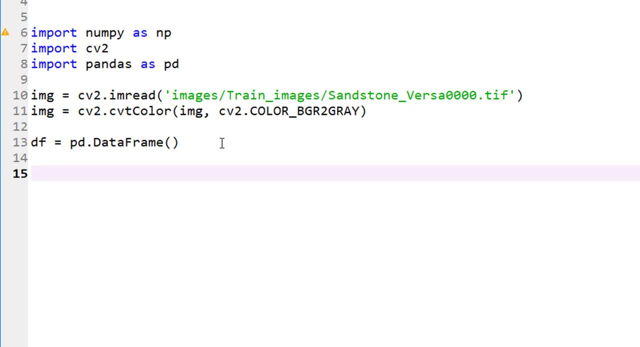 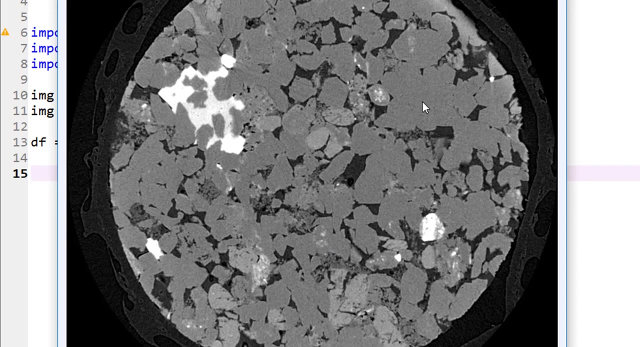 Okay, so this is where, now, We started to engineer our features. Which features do we need for our machine learning algorithm? So feature number one is always. the most important feature would be the pixel value itself. If you look at the image up here, you can see that the pixel value tells us a lot about what it could be. 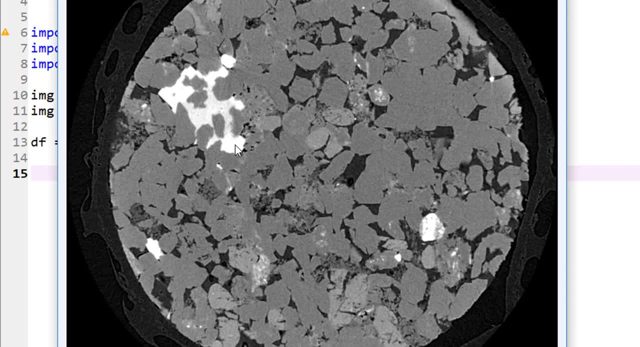 So the bright pixel value, for example, anything above 200, it's a good chance that this is this pyrite or bright phase right here. Okay, anything below- I don't know- maybe 40 or something. This could be this outer area which is air and something else. 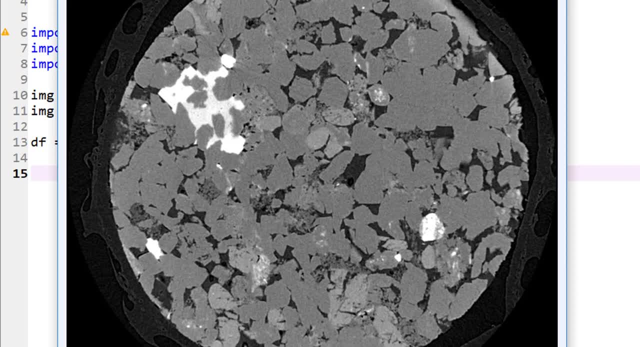 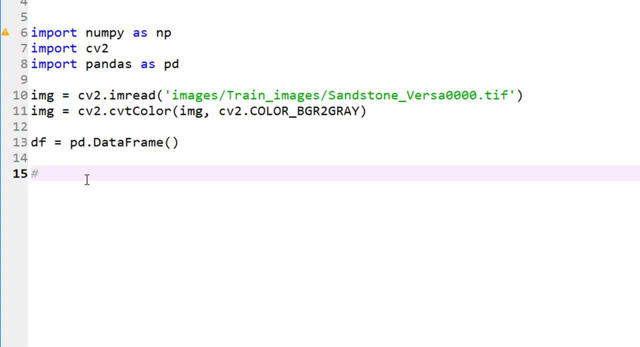 And some sort of an organic stuff out there that's maybe a tape that's wrapped around this sample, Okay, so the feature number one is our original pixels itself. So let's say, add original pixel values, Okay, to the data frame as feature number one. 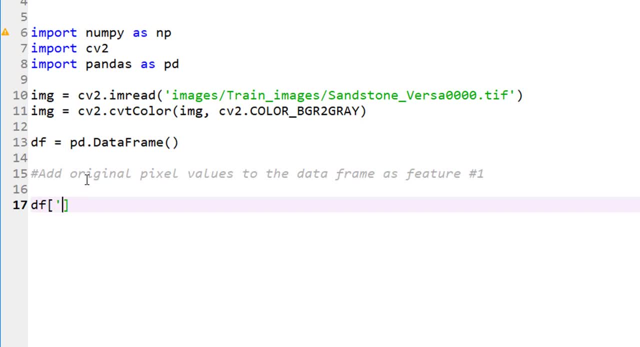 Okay, and how do we do that? Again, to create a new column, you just call the data frame- In our case it's df- and label it. So I'm going to call this original, let's say image, or original pixel values. 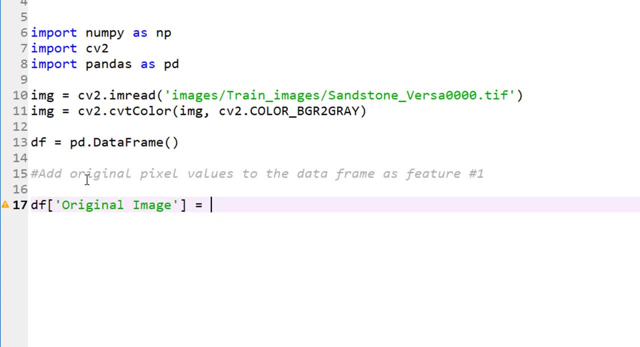 That would be too big of a name, So let's just go ahead and do that now. Pandas is almost like Excel for Python, right? I mean, it's probably not right to say that, But again, for those of you who do not know Pandas, you know it's kind of think of it as Excel for Python. 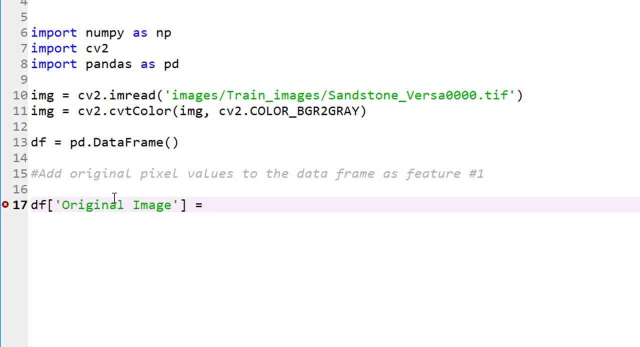 So what do we have in an Excel sheet? We have columns and rows, So original image. This is one of my many features that I'm going to add. So this is, let's say, my column number one. So I'm calling it column number one. 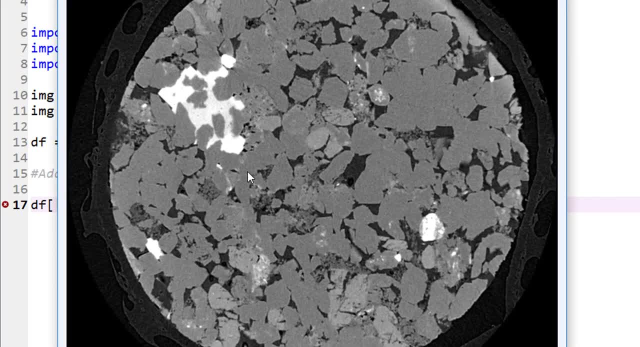 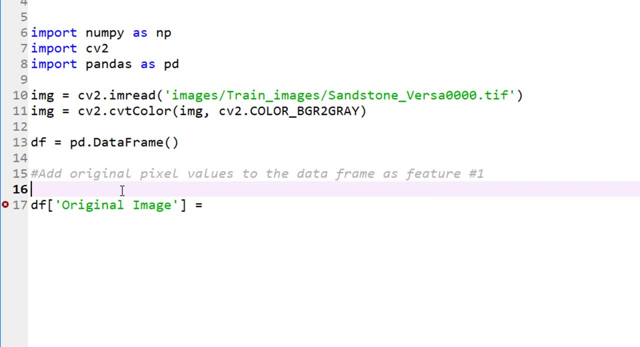 But if you look at the image, this is obviously a 2D image, right, Two-dimensional image. How can I add that in like one column? Basically, what I'm trying to get to here is: you cannot do add this two-dimensional, you know- matrix into one single column. 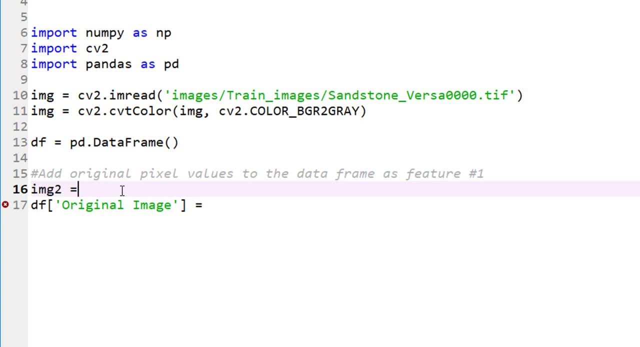 So we have to unwrap it. So I'm going to define a new parameter called image two, which is nothing but reshaped image one or image OK. when I put minus one here, that says: basically reshape my image into single column. That's pretty much it. 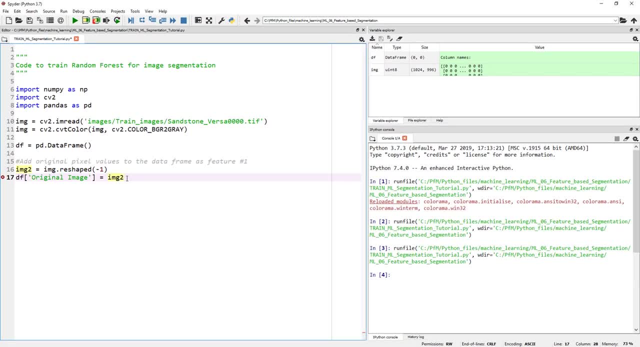 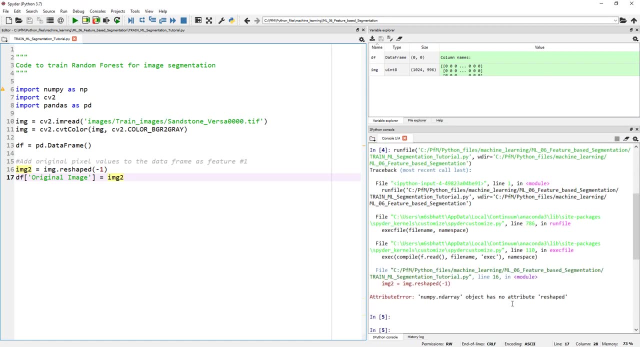 And now I can just add image two pixel values as the row values for my original image. So if I run this again, sanity check it says OK, has no attribute, reshaped. That is because it is just reshape. OK, it's a. 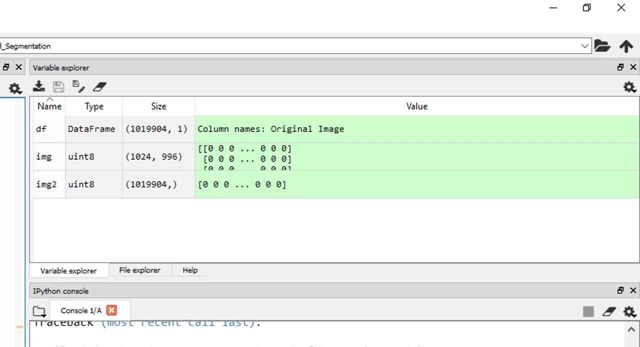 Typo. Now let me go ahead and run it. There you go. So if you look at the variable explorer on the top right here now, my image two is nothing but 1024 multiplied by 996.. That many that you know entries. and my data frame has one column and the column name is original image. 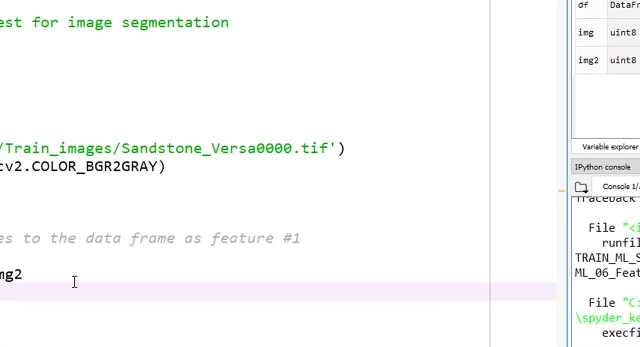 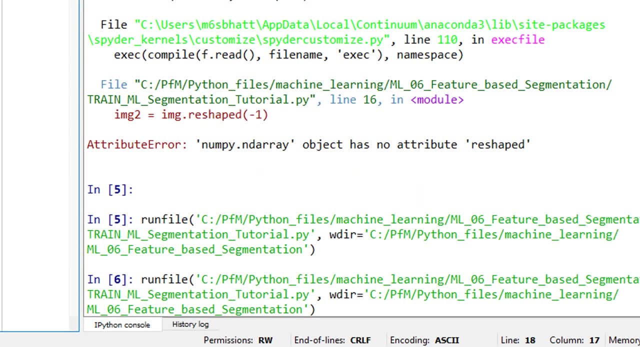 OK, let's go ahead and have a look at it. OK, print data frame dot head, which prints the top Five rows. OK, so there you go. So the top five rows is nothing but all zeros, which is still fine. 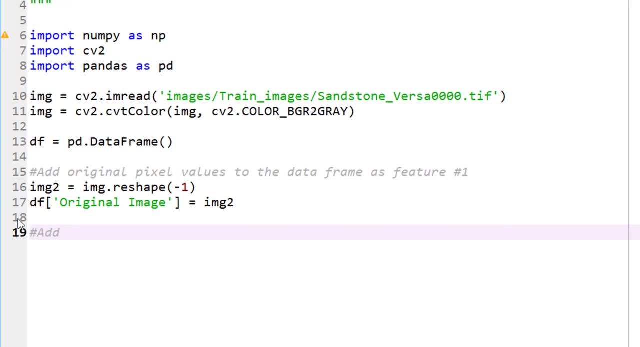 This is a sanity check there. So now, what do we add? Add other features. OK, let's start adding other features. Well, actually, yeah, that's fine, Add other features. So first set would be Gabor. OK, this is my most favorite features. 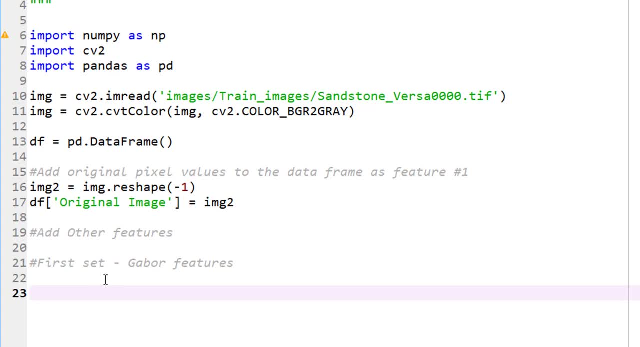 Again, I'm not. I'm just going to repeat everything in this tutorial because I've already done it And I hope I have done a good job in the original video where I talked about Gabor features, which is literally the one before this video, or two before this video in the in the playlist. 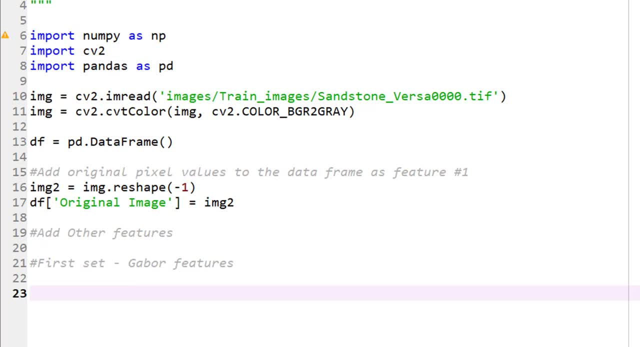 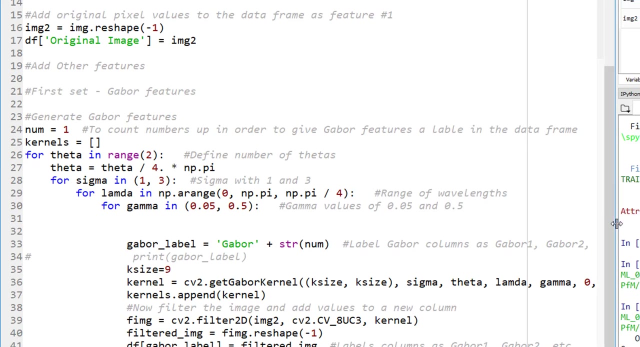 So let me open that other file and copy the code. So I'm copying all of these lines from the other code and pasting it here. Go ahead and save it Now. let me explain for those Of you who are a bit lazy to watch my video, at least right now. let me quickly summarize this. 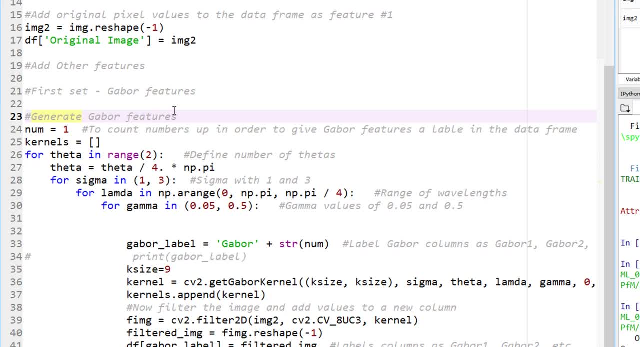 So this is nothing, but it generates a whole bunch of features from the original image by applying various Gabor filters. OK, a Gabor filter is think of a filter such as Gaussian filter or other type of canny edge detection filter or any of those filters. 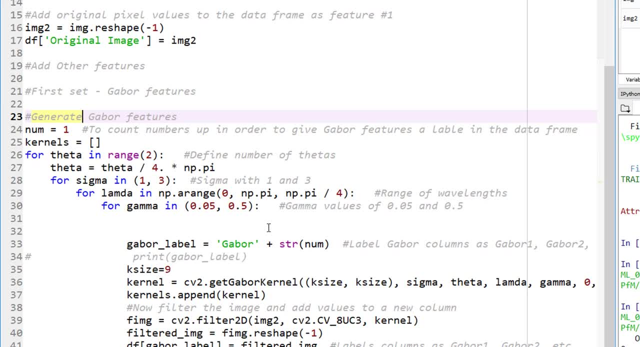 Right. So all you're trying to do is define a kernel and running the kernel onto your image to generate a response from from this convolution. So that's exactly what I'm doing here. All I'm doing is, first of all, look at the kernel itself. 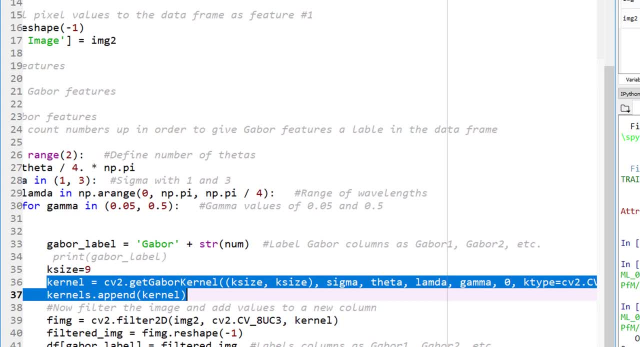 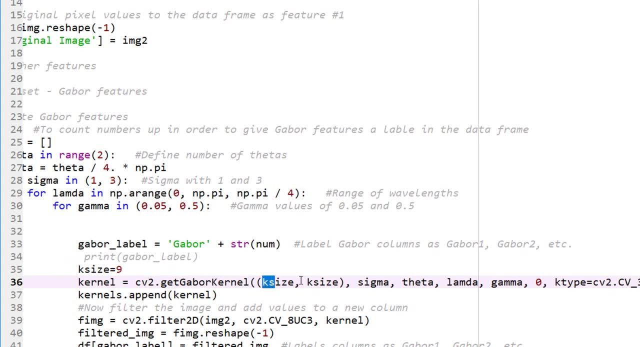 OK, so this is the Gabor kernel. Let me decrease or make more room so you can see it. OK, so the Gabor kernel is nothing, but it has a kernel size which I defined- as if I can see up here where is the kernel size- as nine. 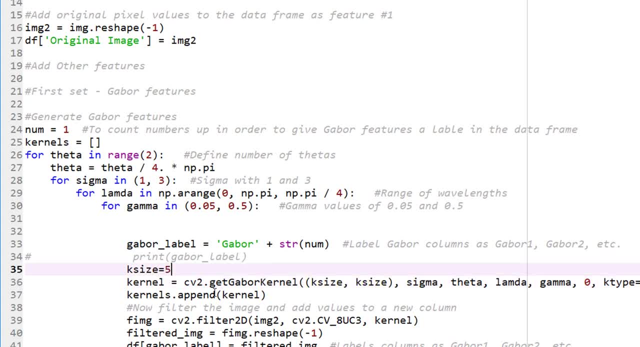 Yeah, this is a nine by nine. In fact, let's change it to 55 gives a better one for our image. So the kernel size is K size and another parameter is sigma. and I'm changing sigma two times here. zero and two. and I'm changing theta. how many times by two? right there. 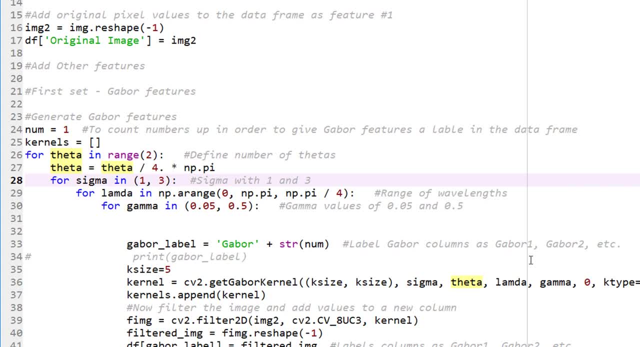 So I'm changing theta, I'm changing sigma with values one and three and I'm changing lambda from zero to pi with a step size of pi Over four, and my gamma is point two or five and point five, OK, point five. point two or five gives, you know, a high aspect ratio kernel. point five gives somewhat a medium aspect ratio kernel. 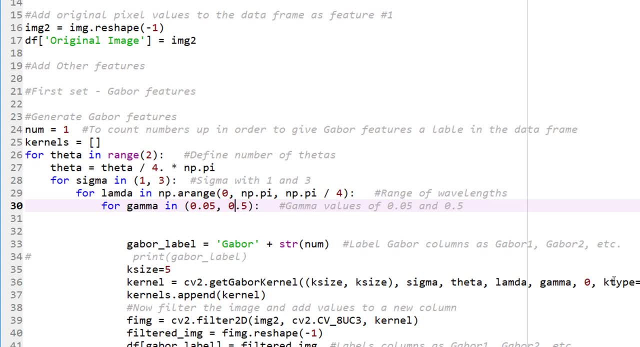 That's why I'm changing that again. I explained it in my video about Gabor. So this code is nothing, but it changes. theta generates a Gabor kernel. changes Sigma generates a Gabor kernel generate. same thing with lambda and gamma. So 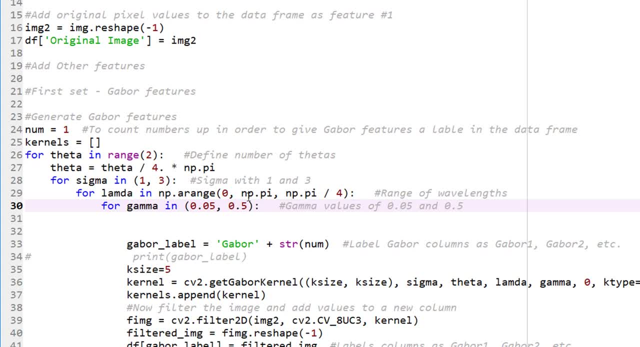 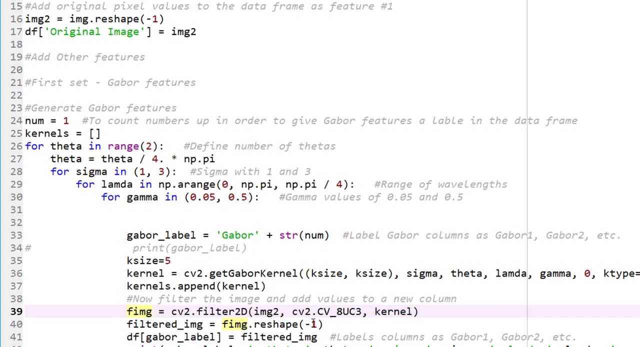 This combination, I believe, gives like 32 different filters and each time a kernel is generated, we are actually running that kernel on image two or applying that kernel on image two. OK, and looking at the response, and now we take that response, or we take the filtered image and reshaping it to minus one because we want to convert that into a column and adding that to my data frame. 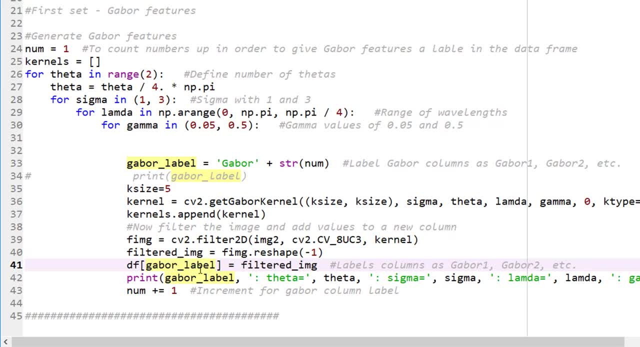 OK, with a label called Gabor label. and what is Gabor label? nothing but the text Gabor plus. whatever that string name is like in this example, the first time would be Gabor one. the second time it applies it would be Gabor two, because I'm increasing number every time it goes through the loop. 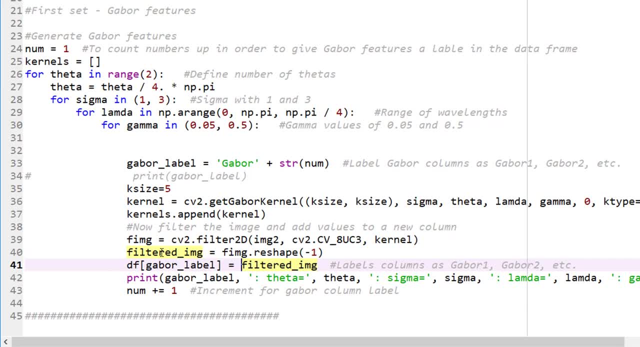 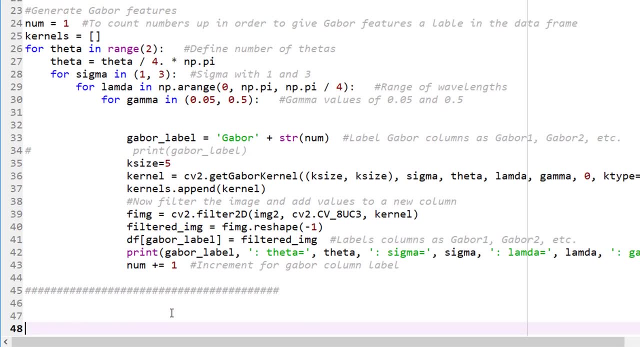 That's it OK. go ahead and study this code. but this is as simple as it gets, OK. so now the next step: let's actually go ahead and print our data frame to see If it is doing what it is supposed to. 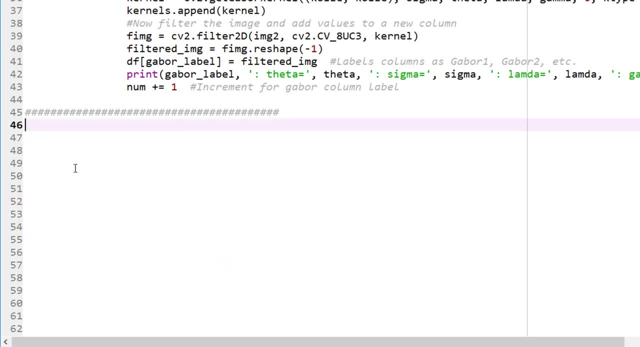 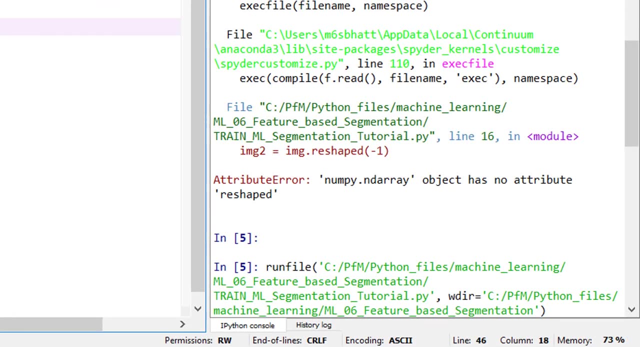 OK, let me create a bit of a room here and now let's go back here. OK, so I'm going to print the same thing: D, F, dot head. Now we should see more columns, OK, so let's go ahead and run this and let me expand this side so you can see it. 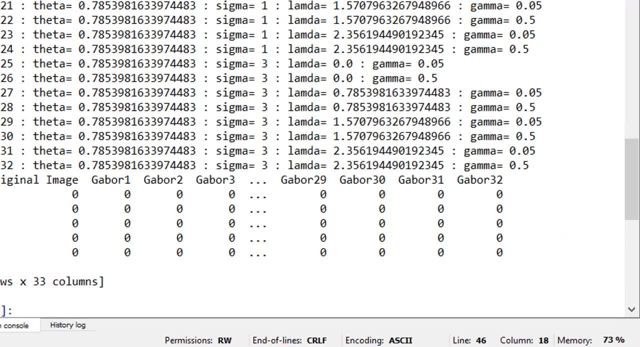 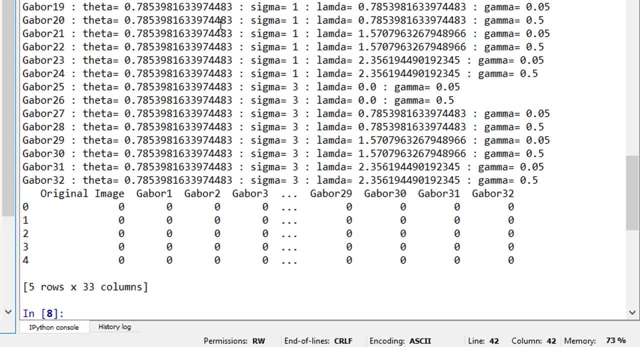 OK, so it looks like while it's working, I'm actually printing the Gabor. wherever that print statement is down here, I'm actually printing the Gabor label and the values for theta, sigma And others. So this is a good summary, right. 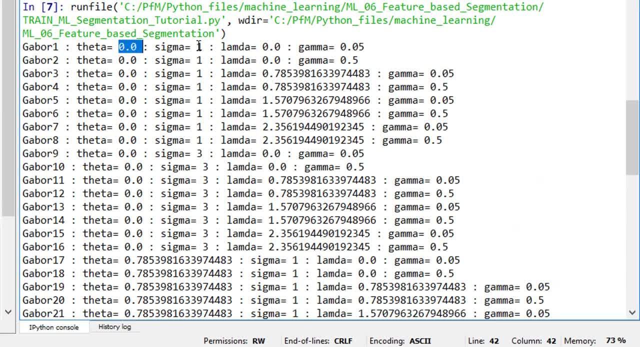 I mean, you can see, the first time, Gabor one is nothing but theta, zero, sigma one, lambda zero, gamma point of five, And then everything else the same except for gamma, And then it goes back to gamma point of five and then changes lambda. 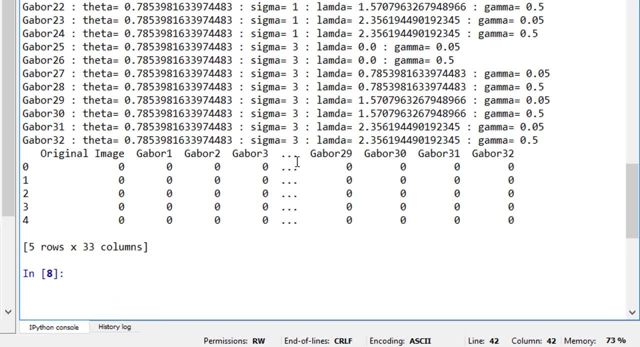 OK and then gamma. So it's going through this loop and you can see my data frame has thirty three columns Now. the first column was the original image and the next thirty two columns are all Gabor responses. I hope that makes sense. 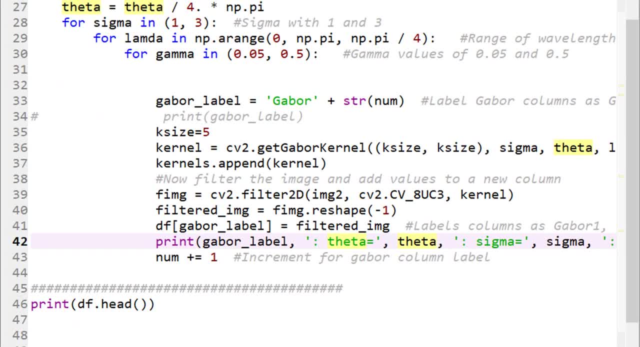 It's nothing, but I'm. I created a Gabor filter bank and just generated a whole bunch of responses by applying the Gabor filter bank like each kernel onto the original image. OK, that's pretty much it. So at this point we can actually go ahead and apply random forest. 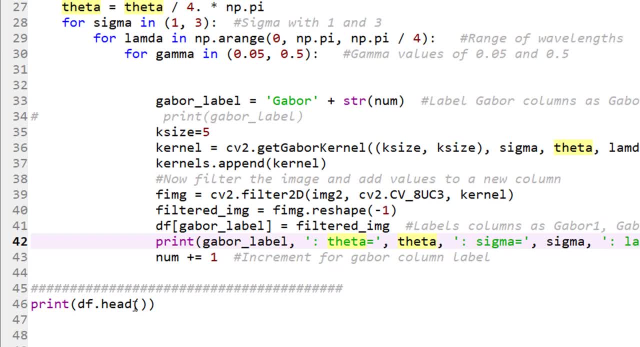 But just for the fun of it, let's add a few other. let's add a few other feature extractors, or filters if you want to call it. So Let's say one of my favorite ones is canny edge, you know so. 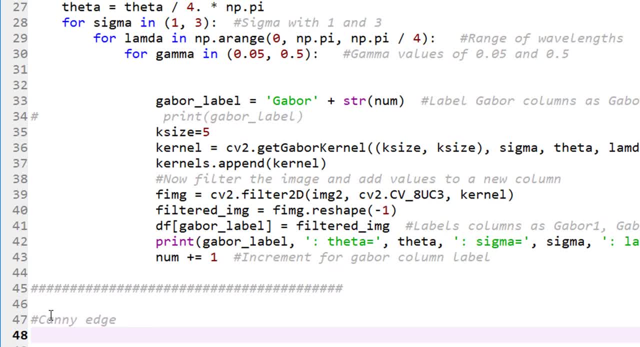 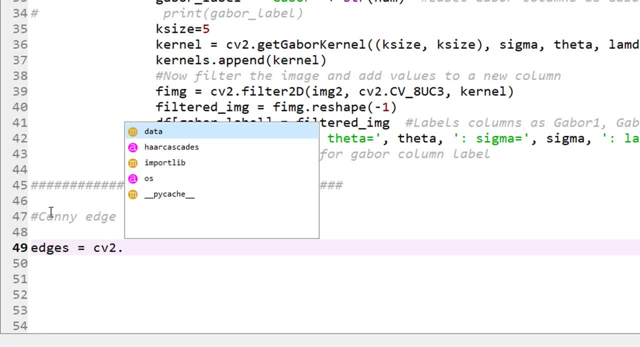 And you probably know what that is. It's again, as the name suggests, it's an edge detection detecting filter, So I'm going to just call this. edges equals to C V two. I think it's an open C V canny. 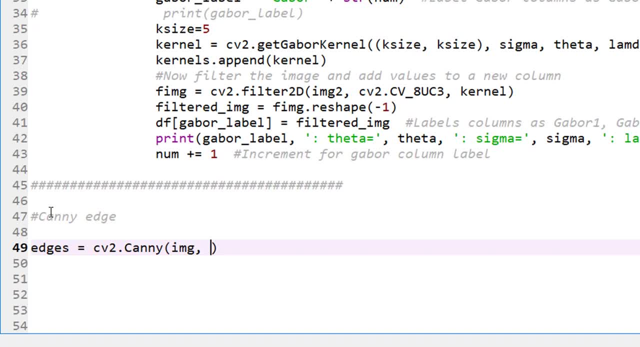 It's very easy to apply. It's just a image and then minimum value and maximum value. Let's just say minimum is 100.. Maximum is 200.. OK, so again you can look at the document. OK, So I'm going to give you a little bit of documentation for this. 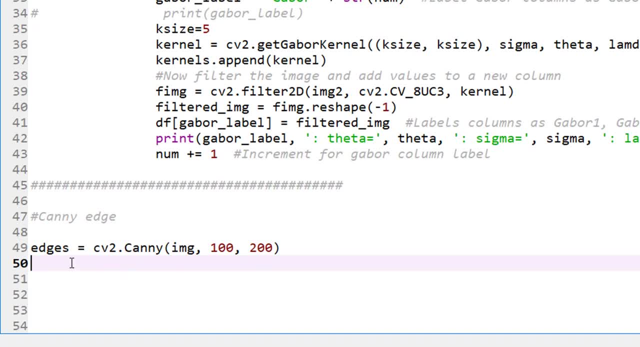 So once this is applied again, I get and canny edged filtered image, but I need to reshape it, So I'm going to just call this edges one equal to edges dot. sorry, reshape minus one. OK, this creates one column and let's add that canny edge. 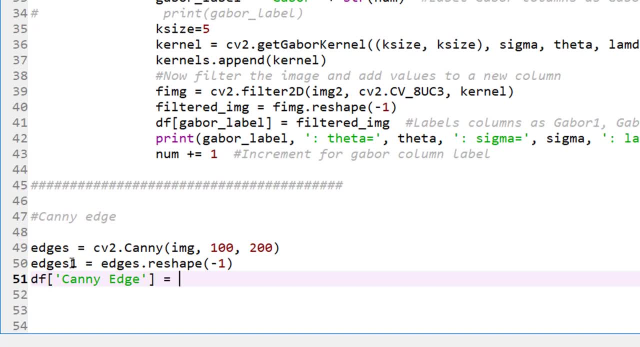 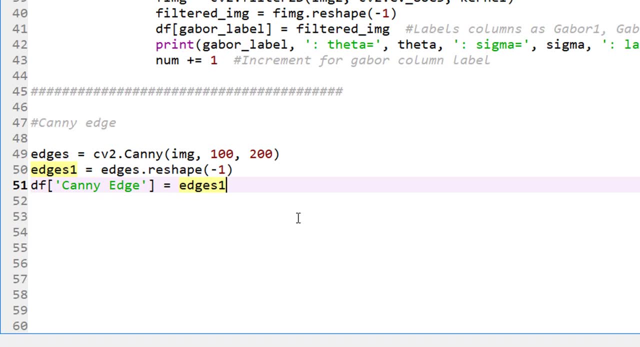 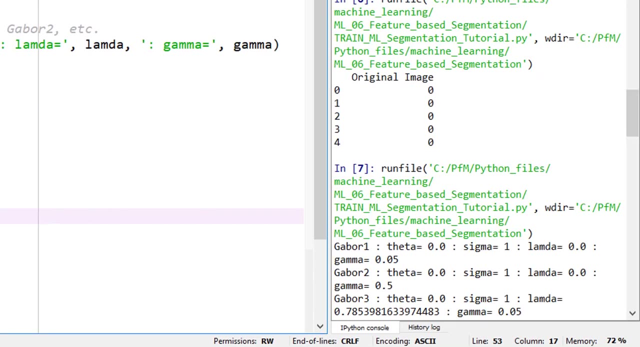 Let's add a column called canny edge and the values are nothing but edges one. OK, I hope that makes sense. So now you can add any number of such filters. Now let's go ahead and again sanity check print data frame dot head. so we can look at the top five columns, run the code and oh, I should have turned that print statement off, but that's OK. 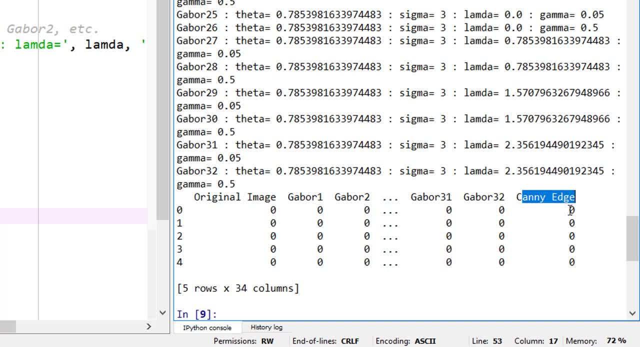 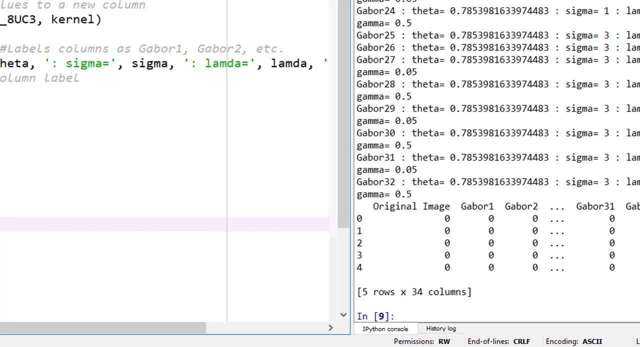 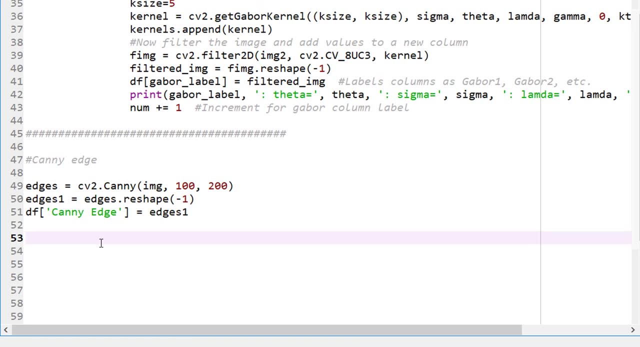 It's fast enough, so we are fine. You see, canny edge column is added right here. OK, let's go ahead and add again. I'm not going to, I'm going to make this video, You know, faster, accelerate this video. but I'm going to add three, four, five or other filters that you can see me type at high speed here. 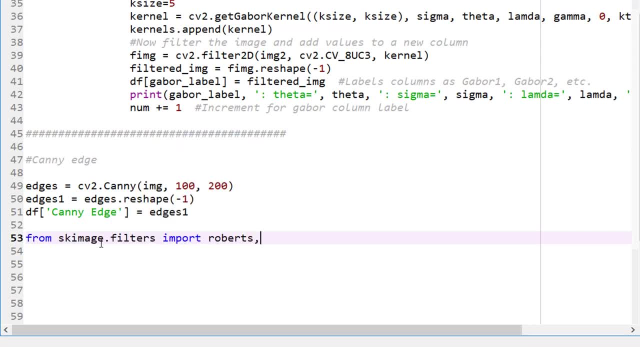 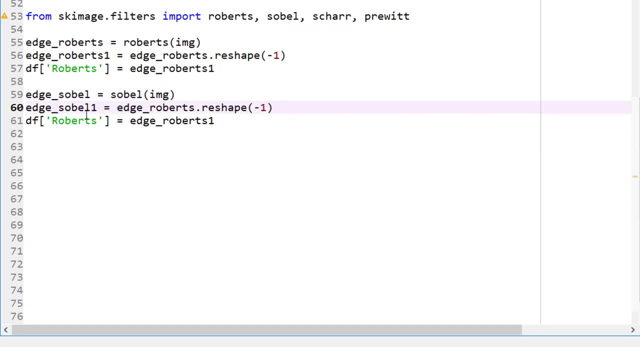 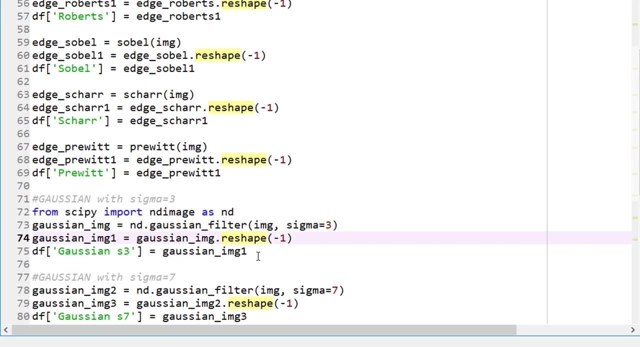 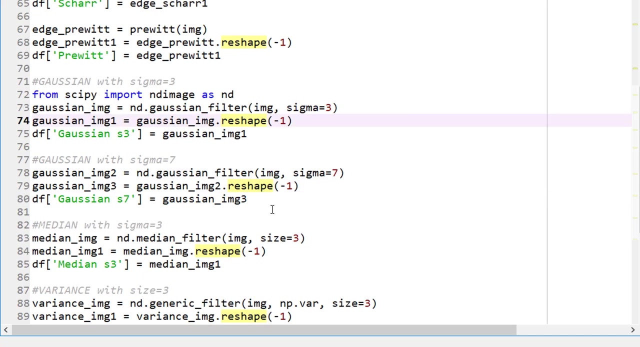 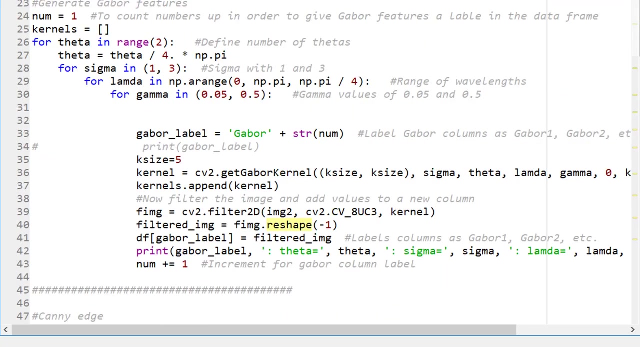 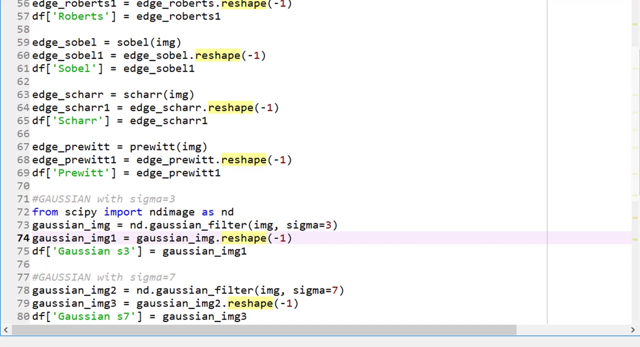 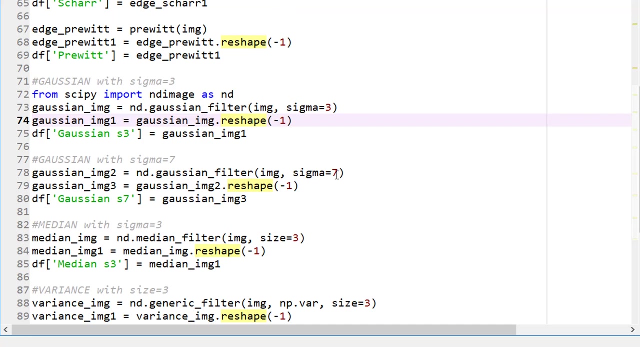 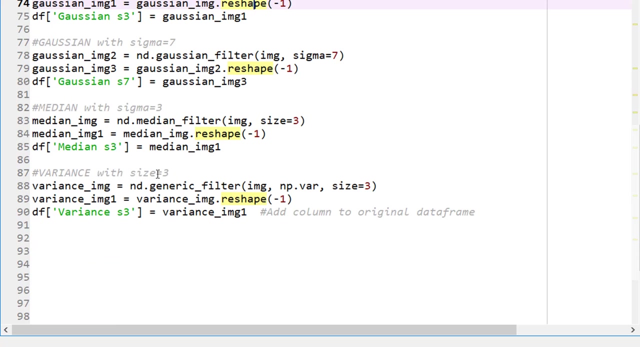 OK, So there you go. So I typed whatever I could and then I copied from other files that I have. So We are actually generating a whole bunch of Gabor filters- in this case like about 32 of them- and the original pixel values, and then we are adding additional columns, each for canny edge, Robert Sobel, Shar Pruitt. Gaussian with the sigma value of three. Gaussian with the sigma value of seven. median with sigma equals to three- you can add more medians if you want- and variance with a sigma size of three. 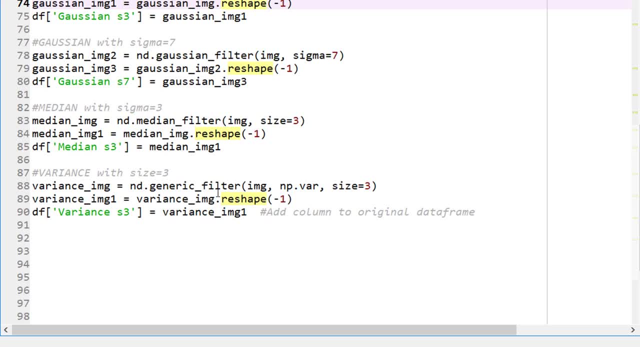 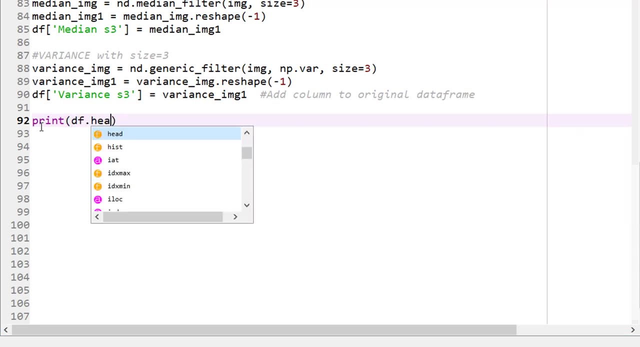 And the way I did. variance is basically: You know, calculated the you know variance using the variance function in NumPy. That's pretty much it, OK. so now final sanity check where we can actually look at print df dot head to make sure everything is OK. 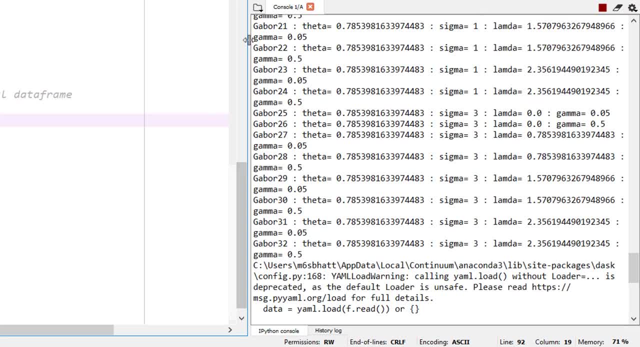 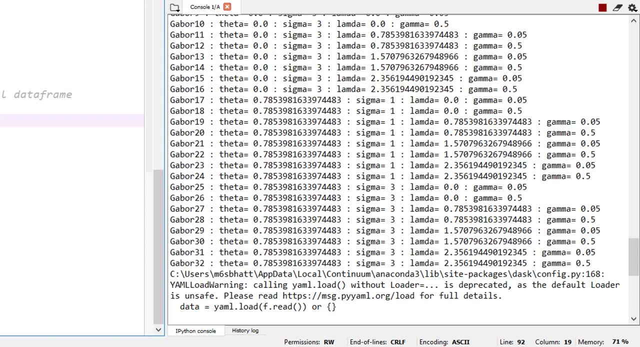 OK, that part is working fine. It's taking its time. I realize that this NP dot, this variance part, is a bit Slow, so if you don't want that, you can go ahead and suppress it, because some of that is actually covered as part of our Gaussian. 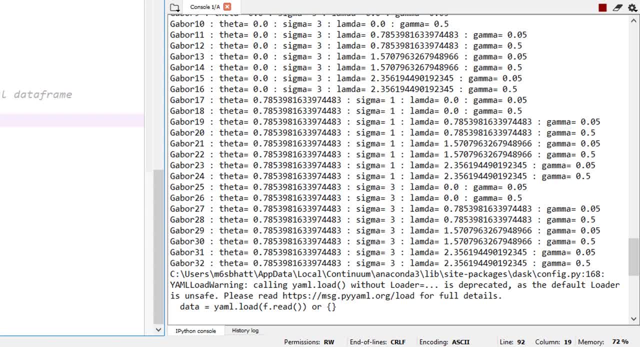 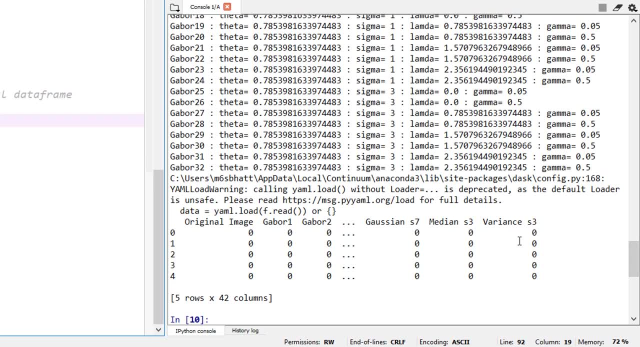 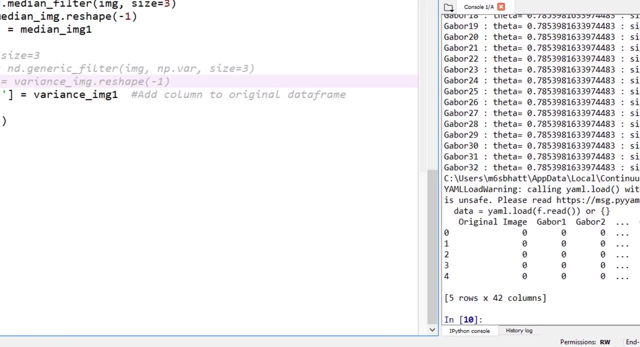 So I mean sorry, Gabor filter, so we may not need that. It's up to you, OK. So there is our, there is our final data frame. and again, if you want to just look at how it is by removing the variance, I bet it would be much faster. 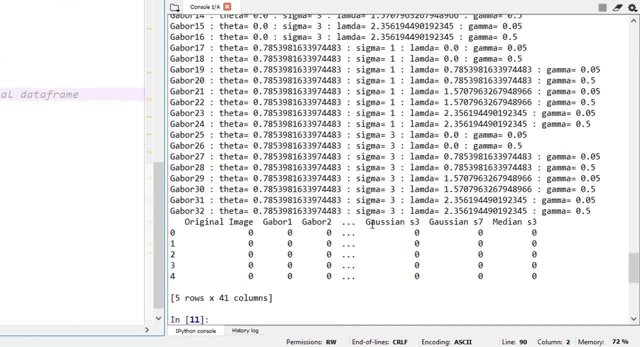 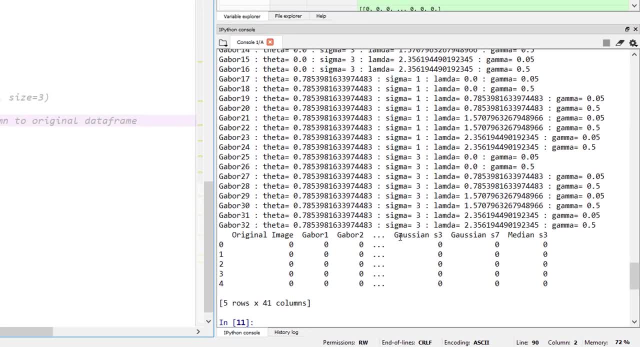 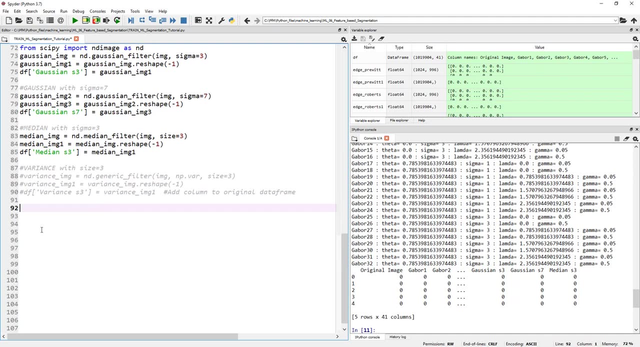 There you go. OK, so let's not worry about variance for now. OK, let's just leave that and continue. OK, so one last step before we move on, which is adding another column, right? I mean, we're not done yet. 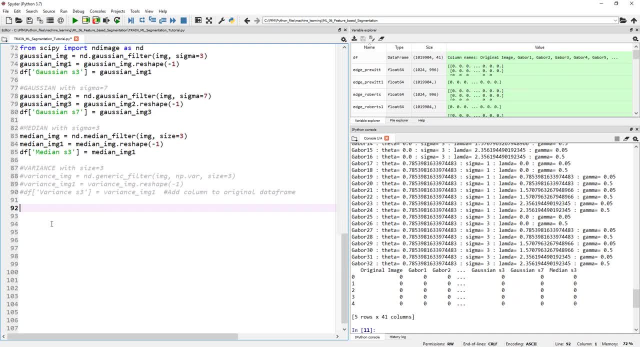 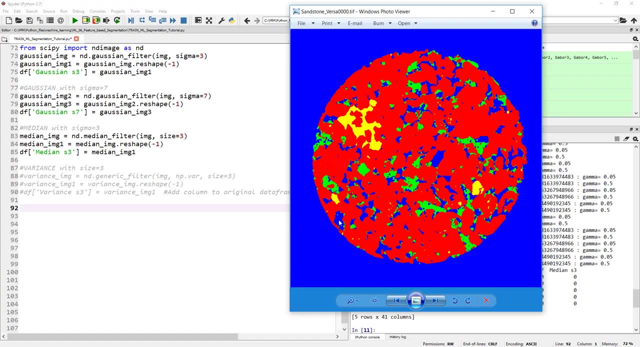 So far we've added all the feature columns. That's it. Now we need to add another column that corresponds to this image. So, now that We have added at every pixel, What is the pixel value? What is Gabor one, two, three, four, five and so on up to 32?? 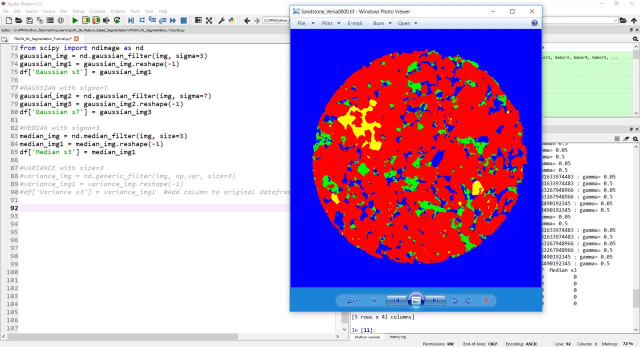 And then what's our Gaussian, The value coming from the Gaussian pixel, filtered image, median image and so on, But we haven't told what the ground truth is. This is by remain. Please remember that we are doing training right, Meaning: we need to tell what the ground truth is. 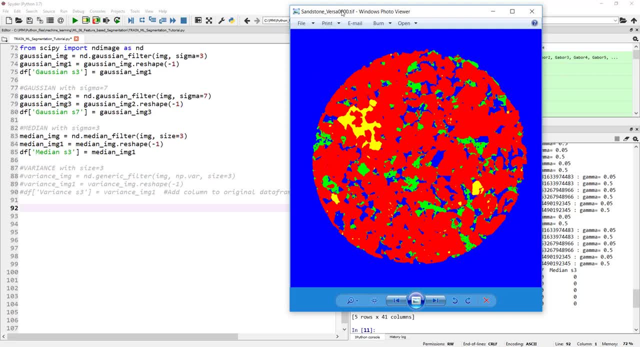 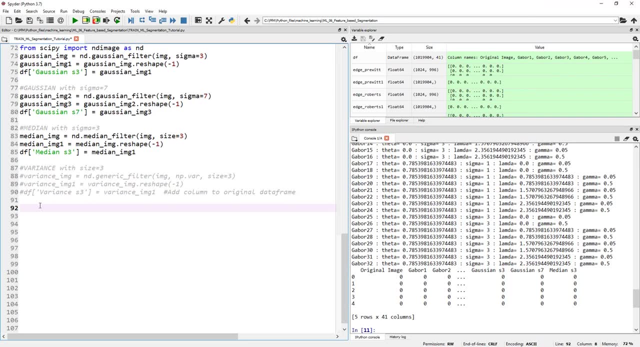 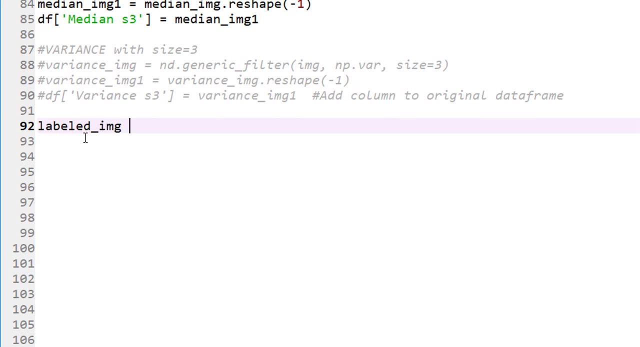 So how do we tell what the ground truth is? Basically, we just read this image, Get the pixel values and then assign to the corresponding row. So how do we do that? Well, exactly as we have done before, So let's just import our labeled image. 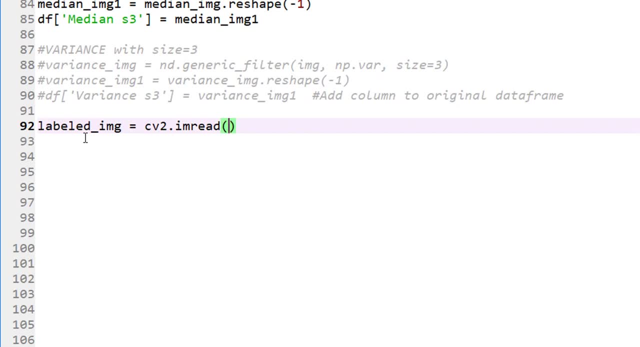 OK, so our labeled image equals to CB two dot in read. OK, and where is my labeled image located? Images- train masks. OK, this is where I stored my labels. I gave it the same name to keep things simple And stone underscore versa one, two, three, four zeros dot. TIFF. 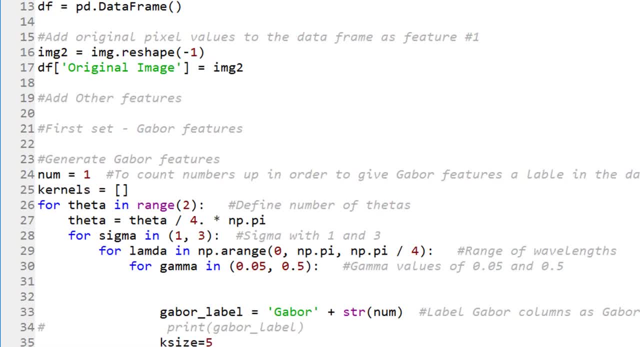 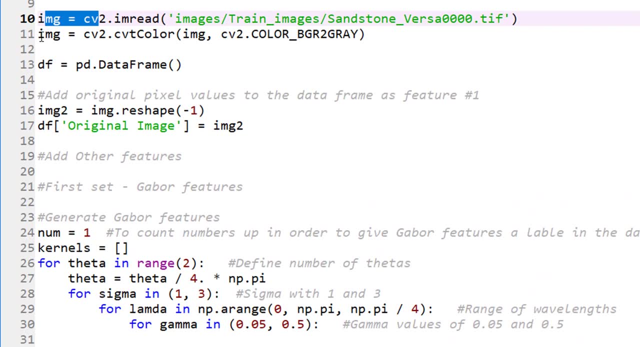 So if I scroll back up, I'm doing nothing different than what we have already done. So this is the original image and I converted that into the gray level here. Let's do the same even for this one. And then we added that to the data frame. 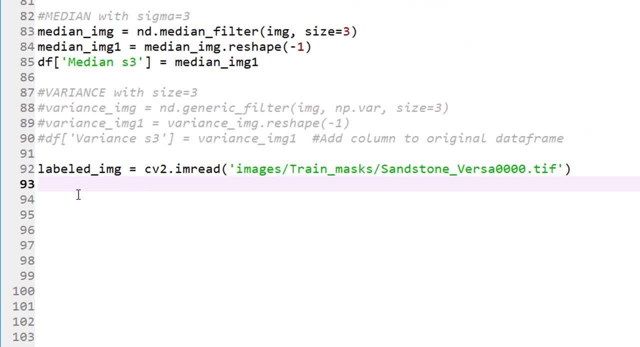 So I'm going to do exactly the same here. So I have my labeled image And I'm going to- I'm going to convert that into a gray image and then reshape it, Right? So sorry, this is not labeled. This is labeled image. 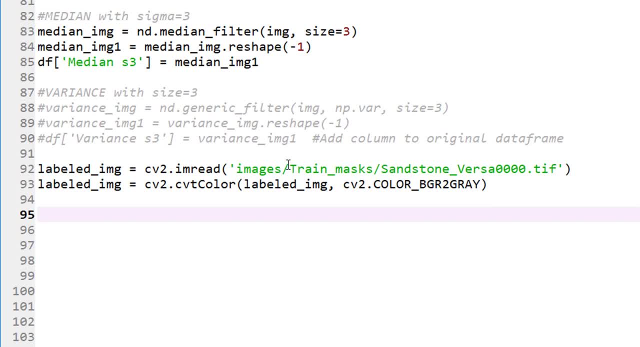 And then all we're doing is convert this red, green, yellow, funky looking image into the gray level image, And we know what the next step is: labeled image one, One equal to labeled image, dot reshape. OK, Again, we are adding a column. 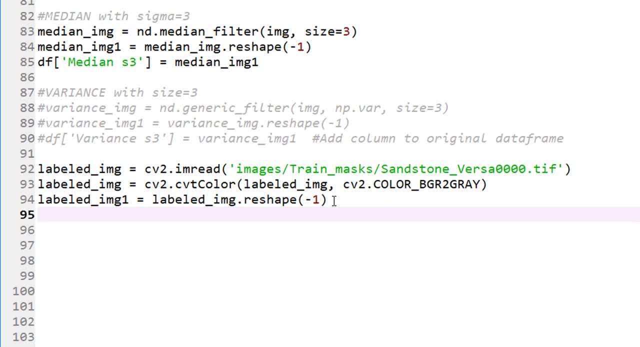 So dot reshape into a single column, And now I can go ahead and add this as the final column, And I'll call this: labels OK Is equal to labeled image one. That's it. So one final time. Print BF dot head. 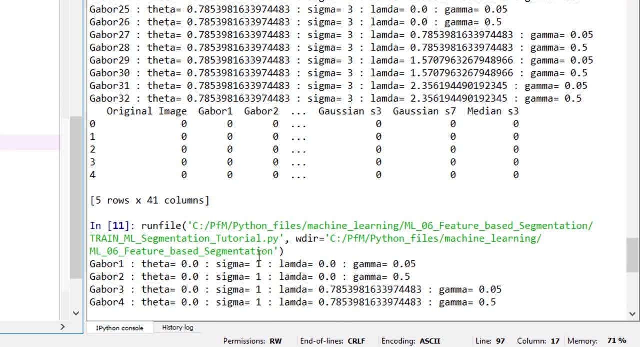 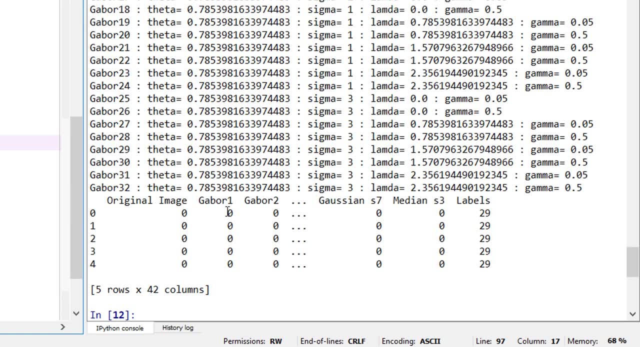 Now we should see the full picture. OK, So these are all different Gabor's, And then for each of this it generates the response, adds it, And then you can see the final value. right there, I mean final column that we just added, which is nothing but labels. 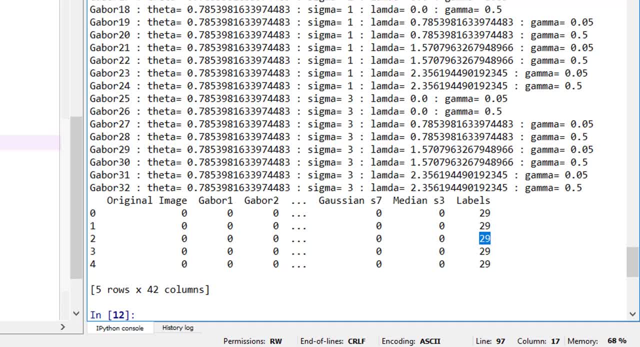 So my labels are 29 and labeled image. I only see 29 here, But there are more labels. You know, 29 is what we see for the first few pixels, which apparently seems to be the best. OK, So I'm going to go ahead and add this to the background pixels anyway.